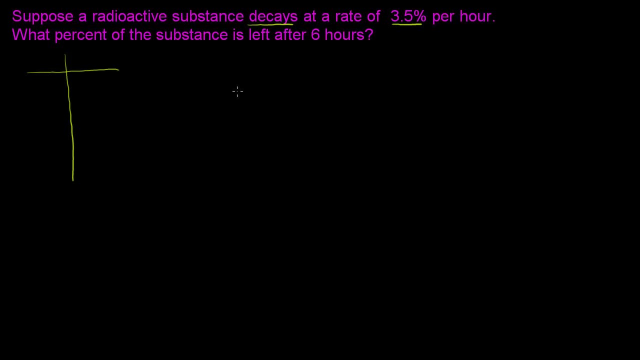 going on and then we'll try to come up with a formula for, in general, how much is left after n hours- So let's say hours that have passed by- and percentage left. So after 0 hours, what percent is left? Well, it hasn't decayed yet. 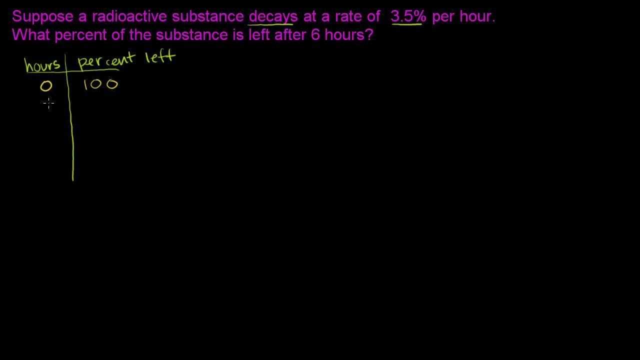 So we have 100% left After 1 hour. what's happened? It decays at a rate of 3.5% per hour, So 3.5% is gone. Or another way, Another way to think about it- is 0.965.. 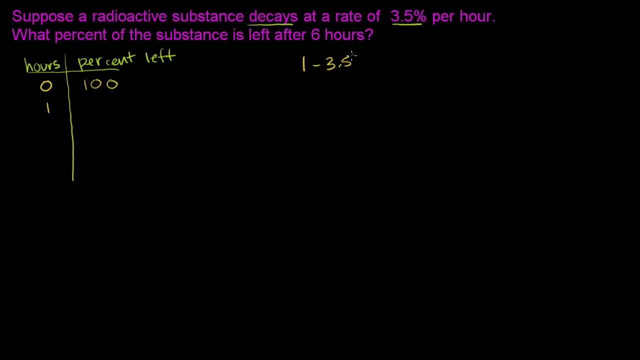 Or remember: if you take 1 minus 3.5%, or if you take 100% minus 3.5%, this is how much we're losing every hour. That equals 96.5%. So each hour we're going to have 96.5% of the previous. 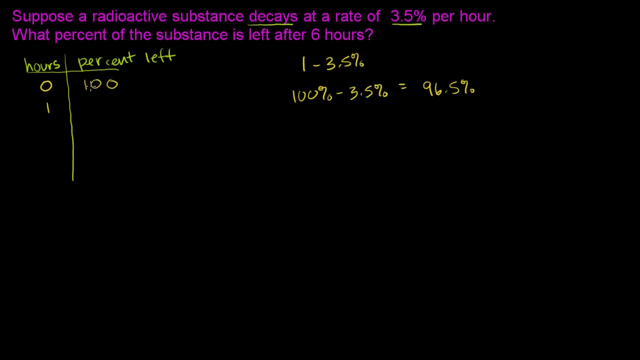 hour. So in hour 1, we're going to have 96.5% of hour 0. Or 0.5%, 0.965 times 100 times hour 0.. Now what happens in hour 2?? Well, we're going to have 96.5% of the previous hour. 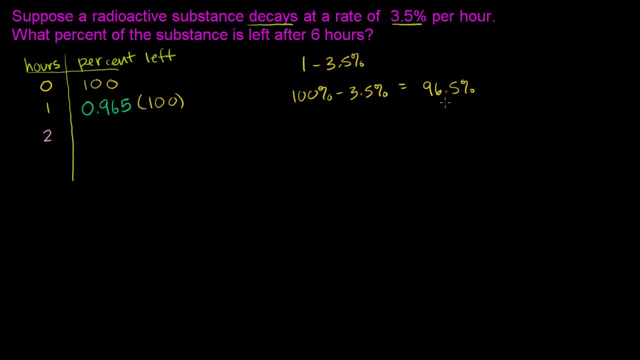 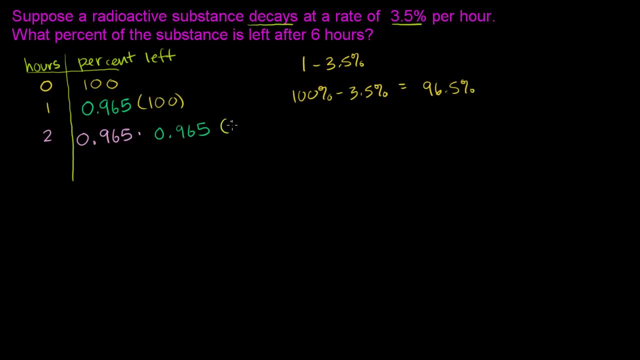 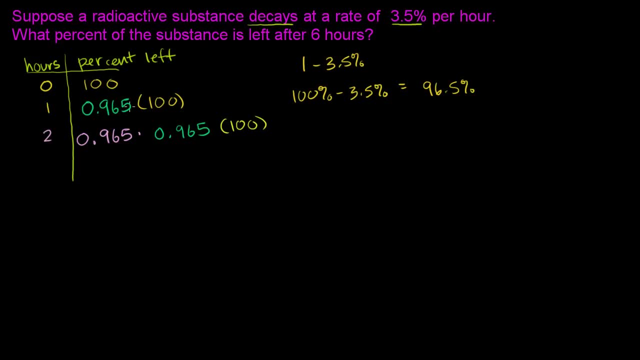 So in the first hour we have 0.965 to the first power times 100.. In the 0th hour we have 0.965 to the 0th power. We don't see it, But there's a 1 there times 100. 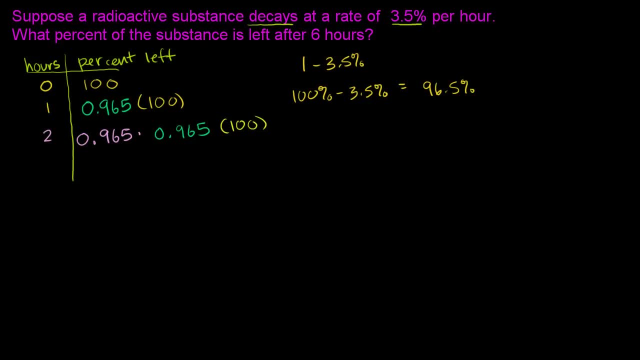 In the second hour, 0.965 to the second power times: 100.. So in general in the nth hour we're going to have 0.965.. 0.965 to the nth power times: 100 left of our radioactive substance. 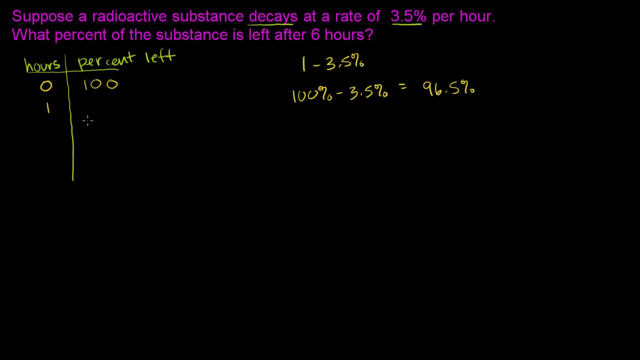 So in hour 1, we're going to have 96.5% of hour 0. Or 0.96.. 0.965 times 100 times hour 0. Now what happens in hour 2?? Well, we're going to have 96.5% of the previous hour. 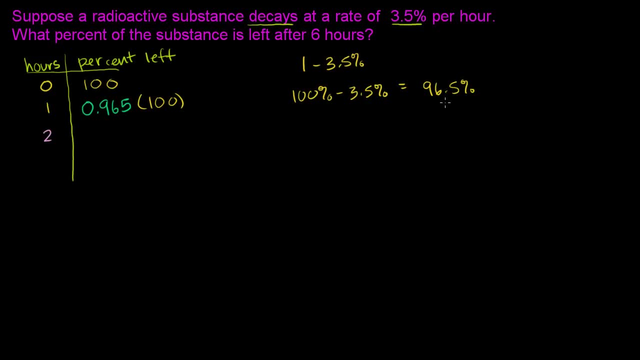 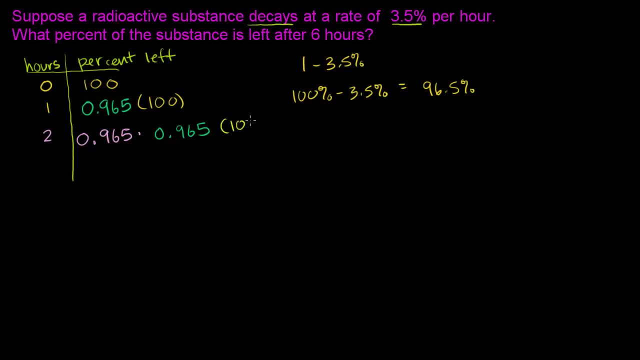 Times 0.965.. Times 0.965.. Times 100.. Times 0.965.. Times 100.. I think you see where this is going in general. So in the first hour we have 0.965 to the first power. times 100. 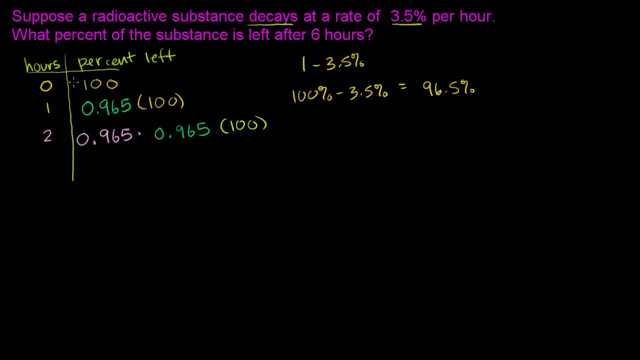 In the 0th hour we have 0.965 to the 0th power. We don't see it, but there's a 1 there Times 100.. In the second hour, 0.965 to the second power times 100.. 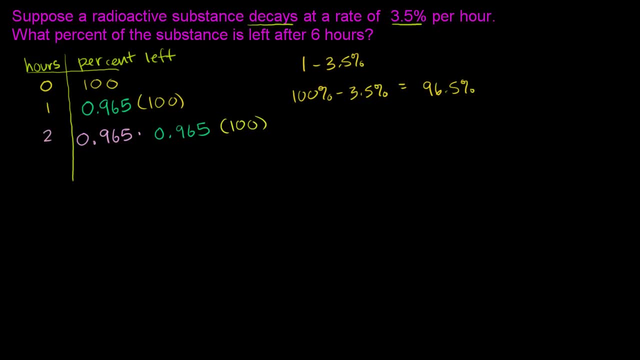 So in general, in the nth hour- let me do this in a nice bold color- in the nth hour we're going to have 0.965.. 0.965.. 0.965 to the nth power times, 100 left of our radioactive substance. 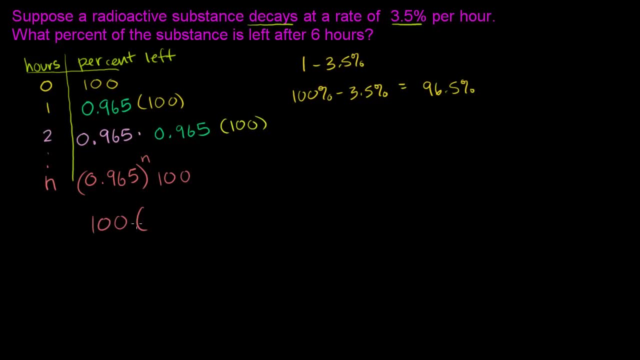 And often times you'll see it written this way: You have your initial amount times your common ratio, 0.965 to the nth power. This is how much we're going to have left after n hours. Well, now we can answer the question. 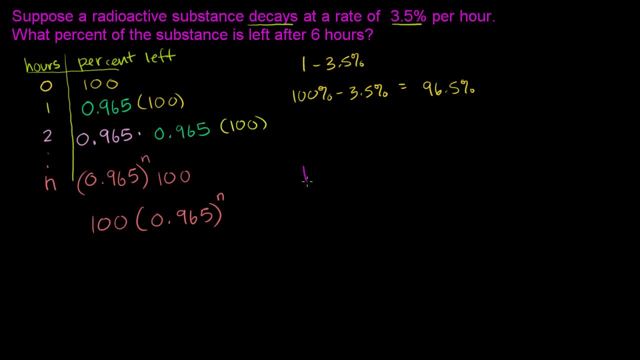 After 6 hours, how much are we going to have left? Well, we're going to have 100 times 0.965.. 0.965 to the nth power, 0.965 to the sixth power left, and we could use a calculator to figure out what that is. 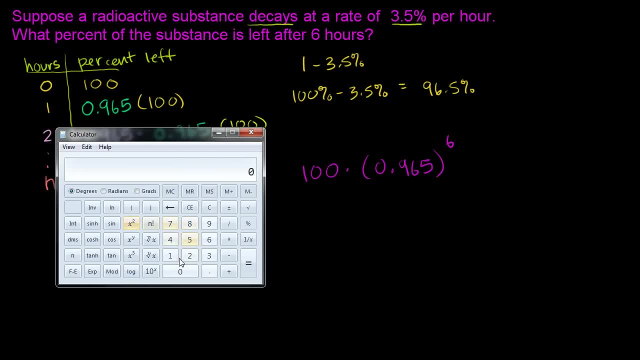 Let's use our trusty calculator. So we have 100 times 0.965 to the sixth, power, which is equal to this is equal to 80.75.. This is all in percentages, so it's 80.75% of our original. 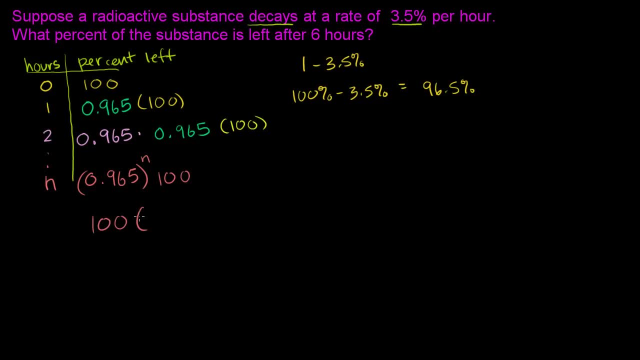 And oftentimes you'll see it written this way: You have your initial amount times your common ratio, 0.965 to the nth power. This is how much we're going to have left after n hours. Well, now we can answer the question. 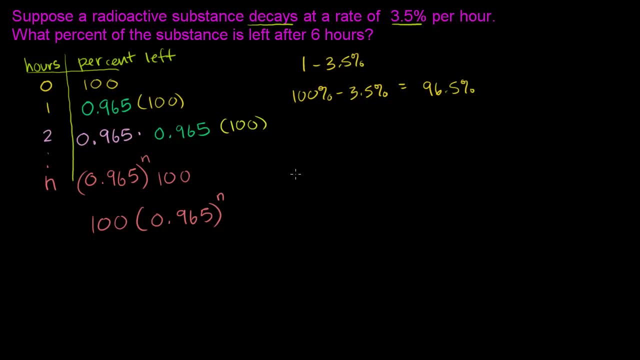 After 6 hours, how much are we going to have left? Well, we're going to have 100 times 0.965 to the 6th power left, And we could use a calculator to figure out what that is. Let's use our trusty calculator. 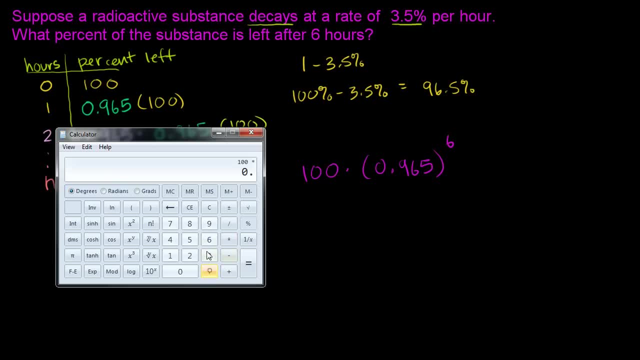 So we have 100 times 0.965 to the 6th power, which is equal to 80.75.. This is 0.965.. And this is all in percentages, So it's 80.75% of our original substance. 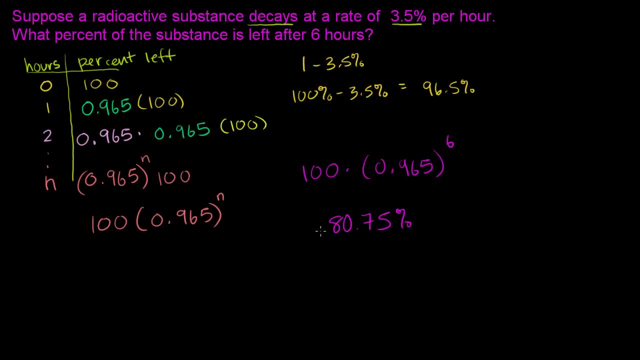 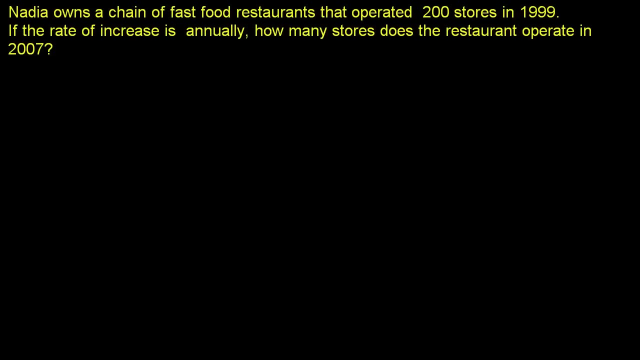 So 80.75%. Let's do another one of these. So we have: Nadia owns a chain of fast food restaurants that operated 200 stores in 1999.. In 1999., If the rate of increase is: Oh, actually there's a typo here. 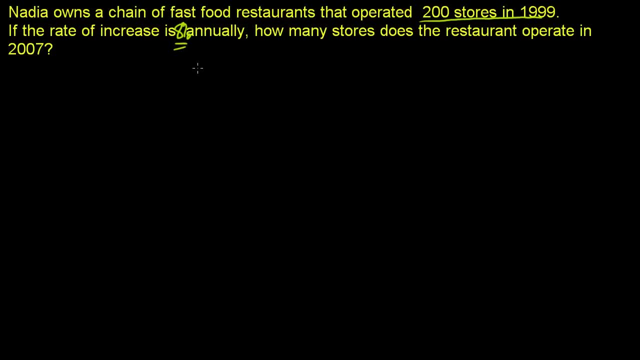 It should be. It should be 8%. The rate of increase is 8% annually. How many stores does the restaurant operate in 2007?? So let's think about the same thing In 1999.. So let's say years after 1999.. 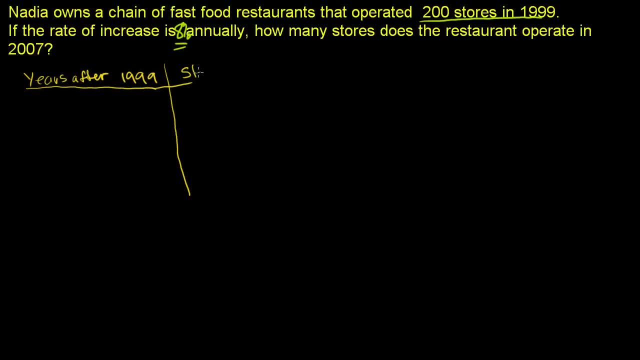 And let's talk about how many stores Nadia is operating Her fast food chain. So in 1999,- 1999 itself is 0 years after 1999, and she is operating 200 stores. Then in 2000,, which is 1 year after 1999,, how many is she going to be operating? 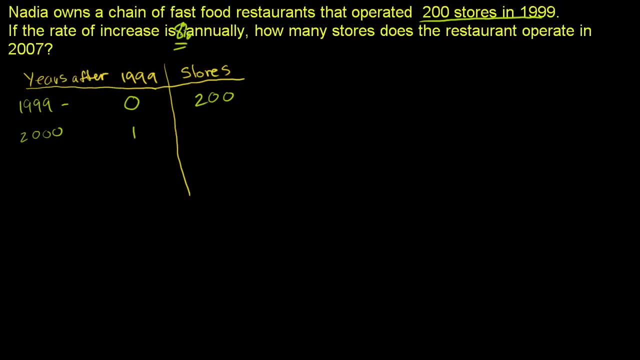 Well, she grows at the rate of 8% annually. So she'll be operating all the stores that she had before, all the stores that she had before, plus 8% of the stores she had before, So 1.08 times the number of stores she had before. 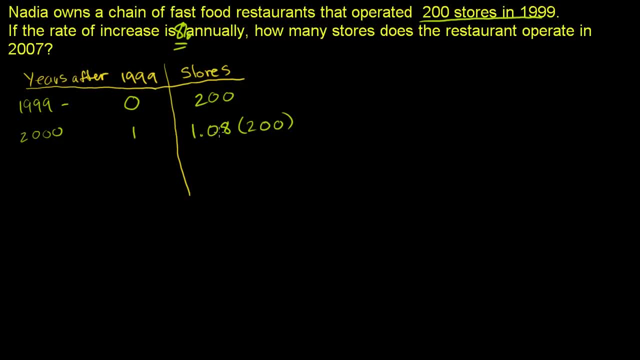 As you're going to see, the common ratio here is 1.08.. If you're growing by 8%, that's equivalent to multiplying by 1.08.. Let me make that clear: 200 plus 0.08 times 200.. 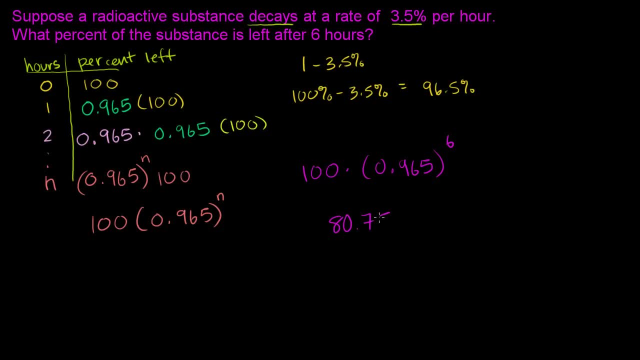 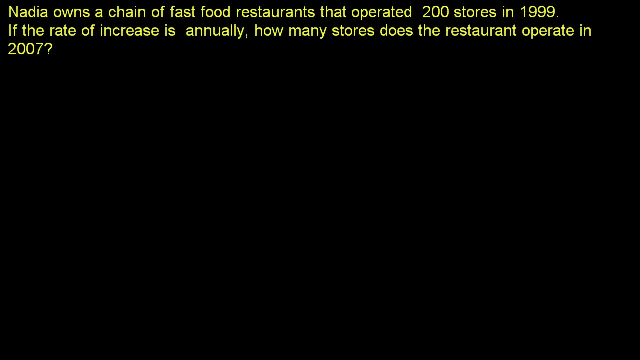 substance, So 80.75%. Let's do another one of these. So we have: Nadia owns a chain of fast-food restaurants that operated 200 stores in 1999.. If the rate of increase is actually- this is a typo here- it should be 8%. 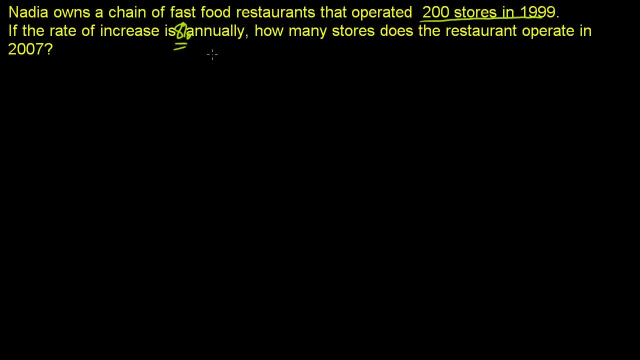 The rate of increase is 8%. How many stores does the restaurant operate in 2007?? So let's think about the same thing in 1999.. So let's say years, years after 1999, and let's talk about how many stores. 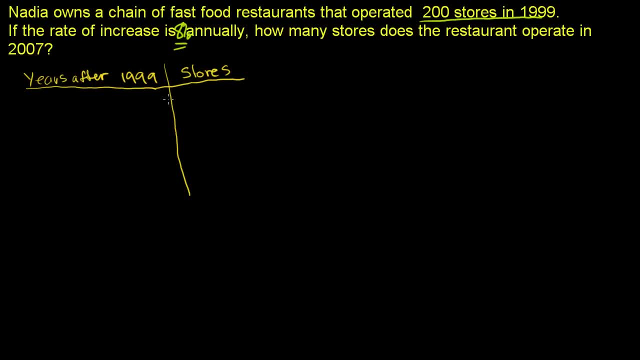 How many stores Nadia is operating her fast-food chain. So 1999, it says, is zero years after 1999, and she is operating 200 stores. Then in 2000,, which is one year after 1999, how many is she going to be operating? 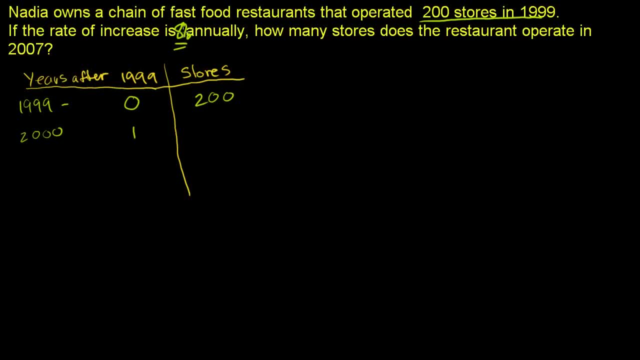 Well, she grows at the rate of 8% annually. So she'll be operating all the stores that she had before, all the stores that she had before, plus 8% of the stores she had before, So 1.08 times the number of stores she had before. 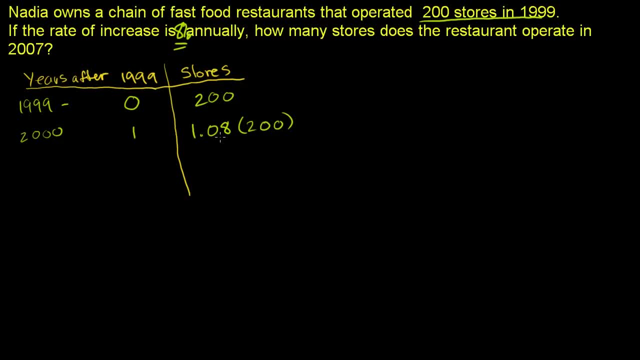 As you're going to see, the common ratio here is 1.08.. If you're growing by 8%, that's equivalent to multiplying by 1.08.. Let me make that clear: 200 plus 0.08 times 200.. 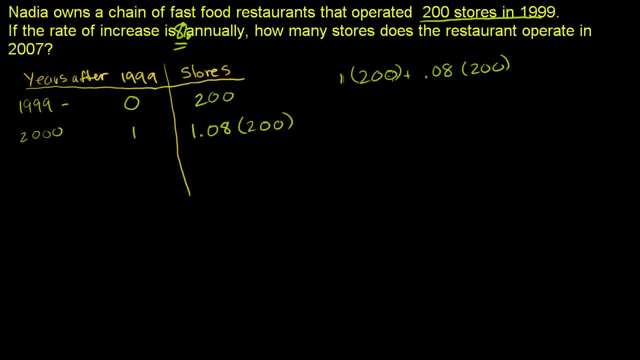 Well, this is just 1 times 200 plus 0.08 times 200. That's 1.08 times 200. Then in 2001,, what's going on? This is now two years after 1999.. You're going to grow 8% from this number. 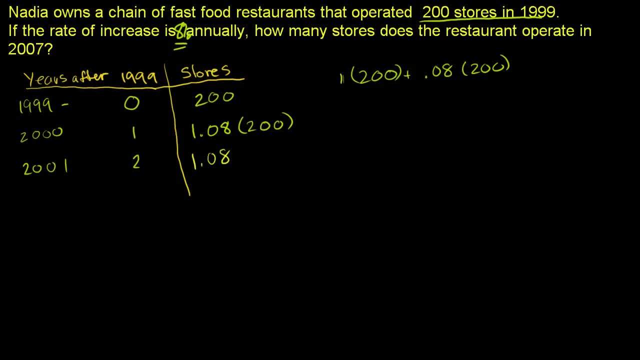 So you're going to multiply 1.08 times that number times 1.08 times 200.. I think you get the general gist If after n years, after 1999, it's going to be 1.08.. Let me write it this way: 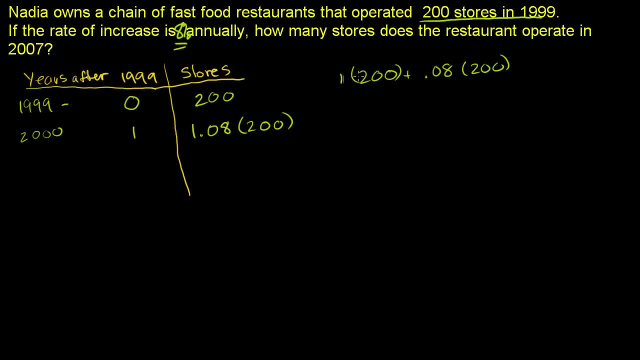 Well, this is just 1 times 200 plus 0.08 times 200. That's 1.08 times 200. Then in 2001. In 2001.. What's going on? This is now 2 years after 1999.. 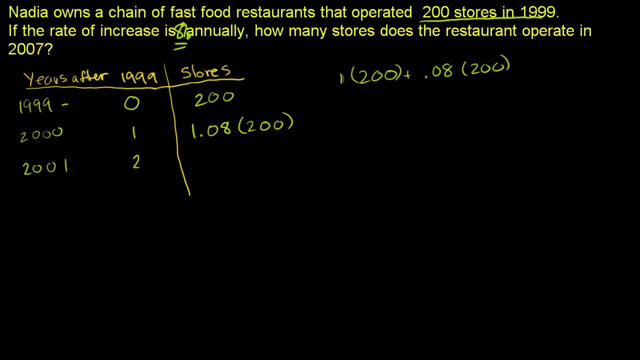 You're going to grow 8% from this number. So you're going to multiply 1.08 times. that number Times 1.08 times 200.. I think you get the general gist If after N years, after 1999, it's going to be 1.08.. 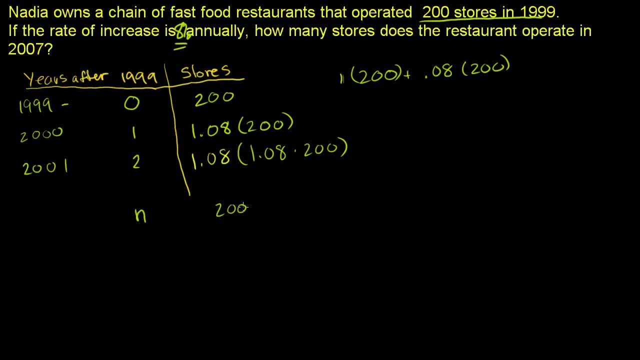 Let me write it this way: It's going to be 200 times 2.08.. 1.08 to the nth power After 2 years. 1.8 squared 1 year: 1.8 to the first power. 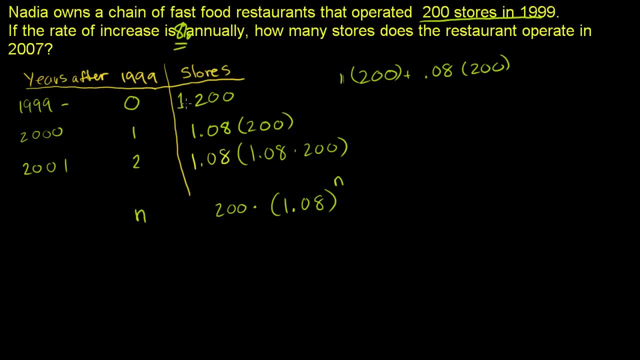 0 years. This is the same thing as 1 times 200, which is 1.08 to the 0th power. So they're asking us: how many stores does the restaurant operate in 2007?? Well, 2007 is 8 years after 1999.. 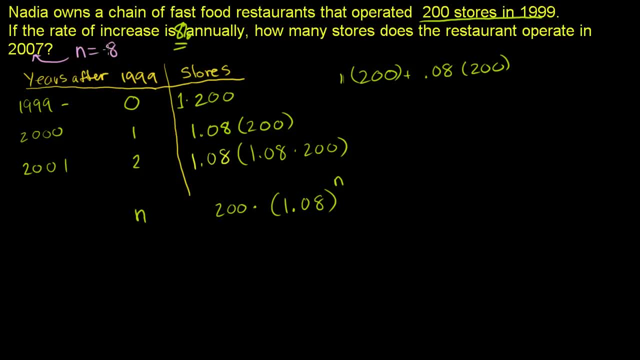 So here N is equal to 8.. So let us substitute: N is equal to 8.. The answer to our question will be: 200 times 1.08 to the 8th power. Let's get our calculator out and calculate it. 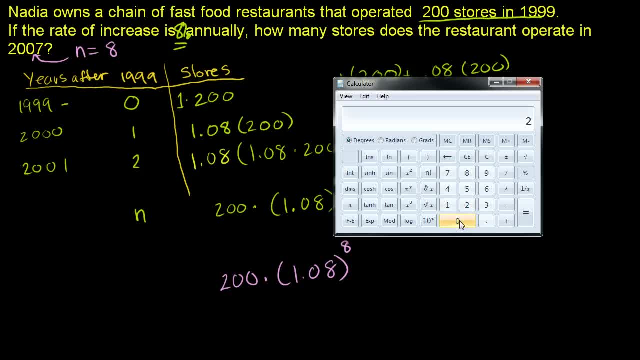 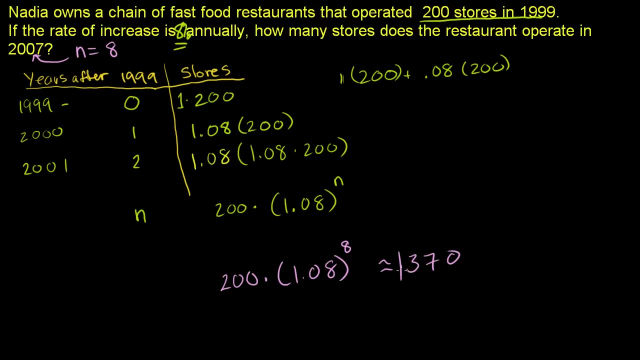 So we want to figure out 200 times 1.08 to the 8th power. She's going to be operating 370 restaurants And she'll be in the process of opening a few more. So she's going to be, if we round it down, she's going to be operating 370 restaurants. 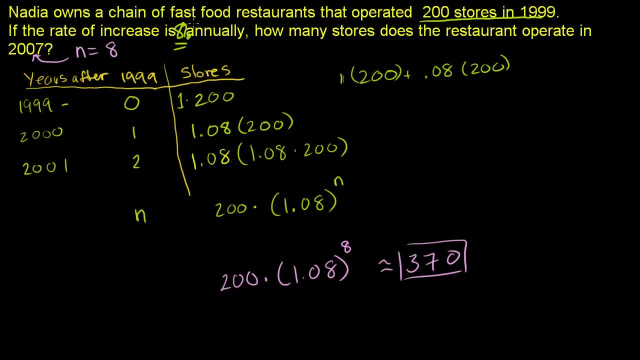 So 8% growth might not look like something that's so fast or that exciting, But in under a decade, in only 8 years, she would have gotten her restaurant chain from 200 to 370 restaurants. So for over 8 years. you see that the compounding growth by 8% actually ends up being quite high.